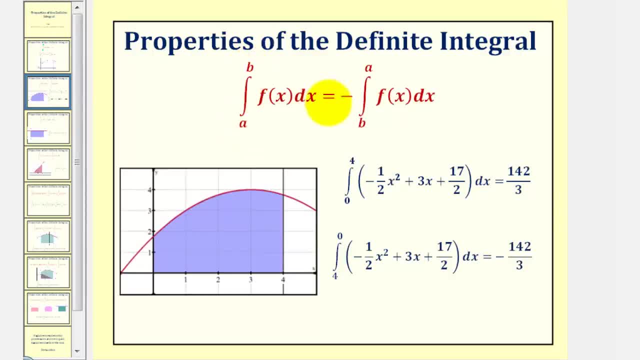 Next we have the integral of f of x from a to b equals the opposite of the integral of f of x from b to a. So notice here, notice here, we've changed the limits of integration. Here we're integrating from a to b, and here we're integrating from b to a. 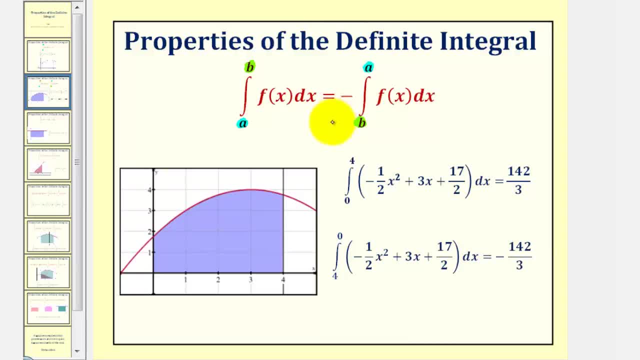 So if we change the order of integration it'll change the sign of the integral Again. as an example, if we integrate our quadratic function here from zero to four, because the function is non-negative over this closed interval, this would give us the area under the function and above the x-axis over this interval. 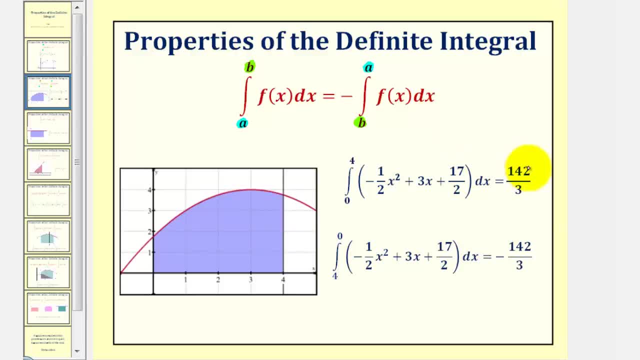 which is this shaded region here which is equal to one hundred forty-two thirds. So notice how we're integrating from zero to four in this direction. And now, if we change the order of integration and integrate from four to zero or in this direction, 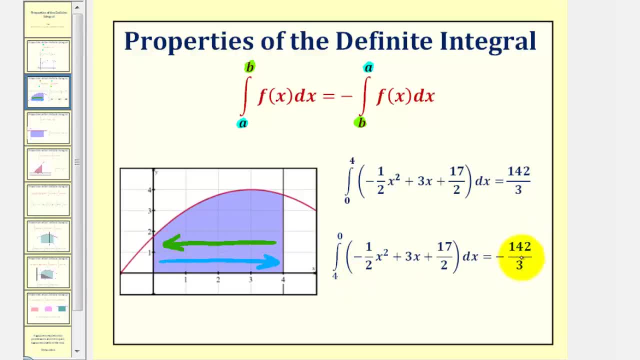 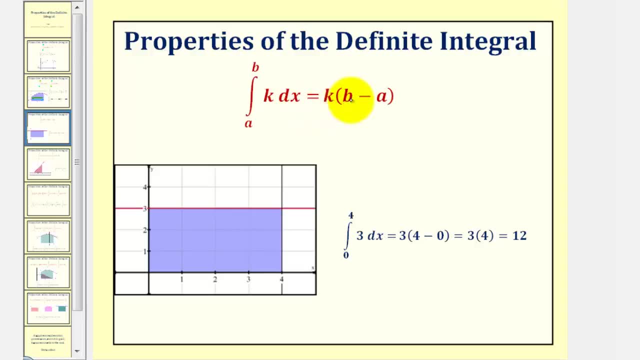 the outcome will be negative one hundred forty-two thirds. Next, if k is a constant, the integral of k from a to b is equal to k times the quantity b minus a. So, as an example, if we integrate three from zero to four, 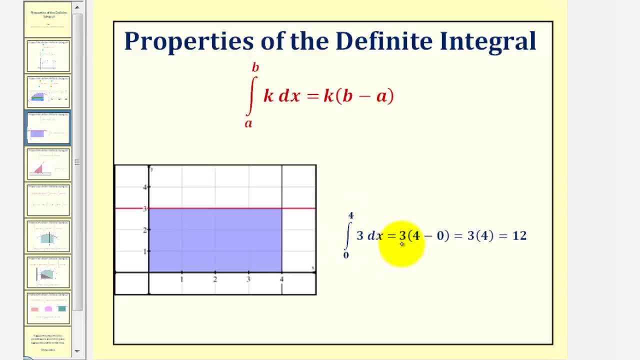 k is three, so this is equal to three times b minus a would be four minus zero, giving us three times four, which equals twelve. And let's see why, If we graph the integrand function f of x equals three. it would be this horizontal line here: 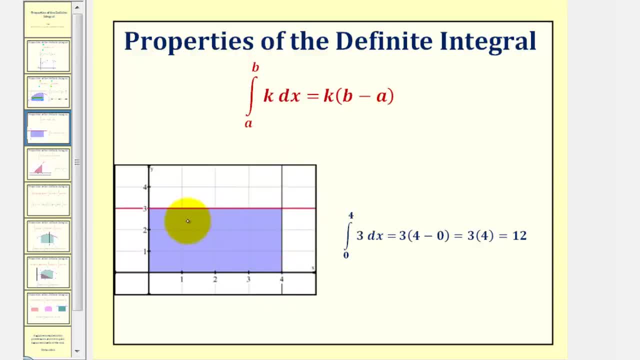 and if our interval is from zero to four, notice how the area below the function and above the x-axis is this rectangle, and we know the area of a rectangle is length times width. So the value of k three actually gives us the length of the rectangle. 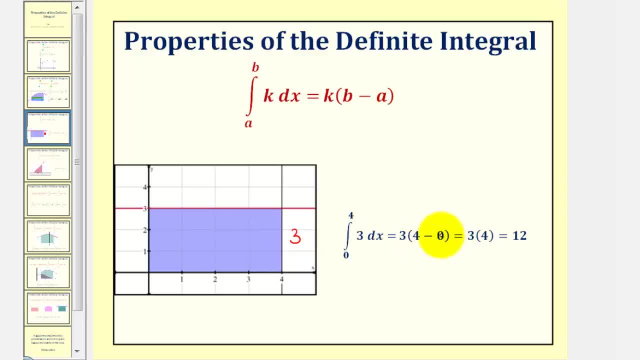 and b minus a, the width of the interval gives us the width of the rectangle, which would be four, giving us a result of three times four or twelve for the value of the def integral. Now, here our constant function is non-negative. 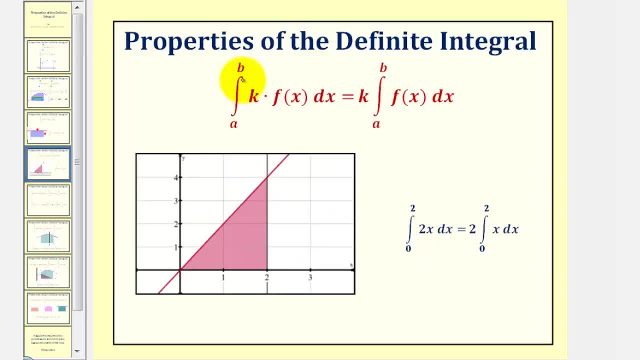 but it doesn't have to be for this to hold true. Next, we have the integral of k times f of x from a to b equals k times the integral of f of x from a to b. So this is telling us that we can factor out the constant k. 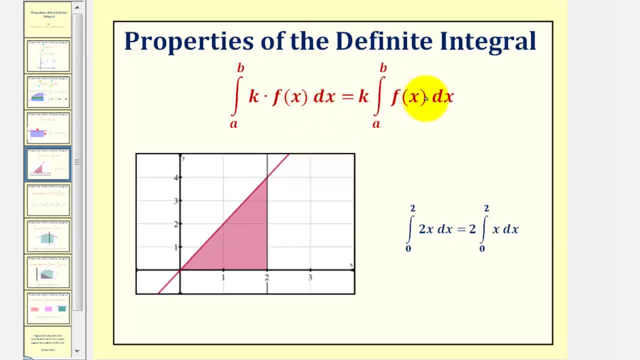 and it does not affect the value of the def integral. So, as an example, if we have the integral of two x from zero to two, we can factor out this two and write this as two times the integral of x from zero to two. 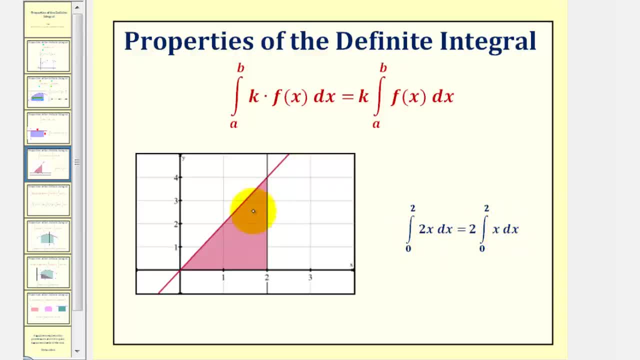 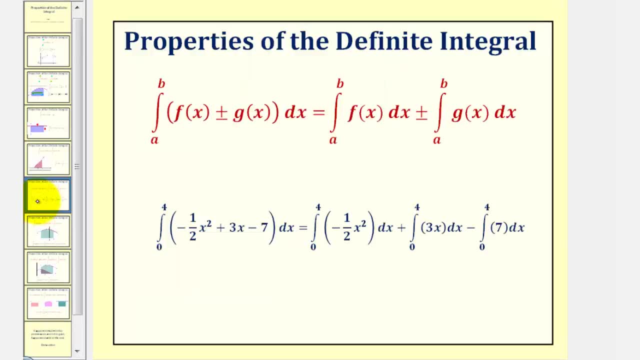 In either case, the value of this def integral would be the area of this triangular region, here Again, because the function is non-negative over this closed interval. Next, we have the integral of f of x plus or minus g of x, integrated from a to b. 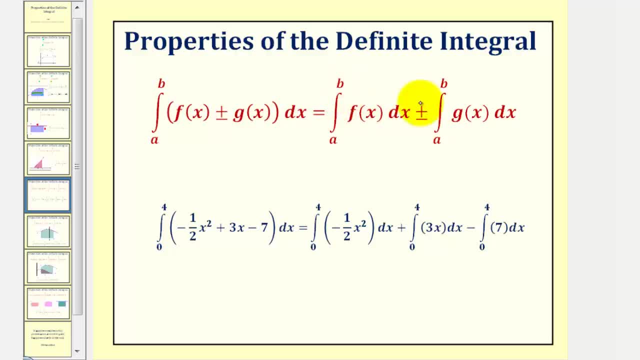 is equal to the integral of f of x from a to b, plus or minus the integral of g of x from a to b. So if we're integrating a sum or difference of functions, we can break it up into separate integrals if we wish. 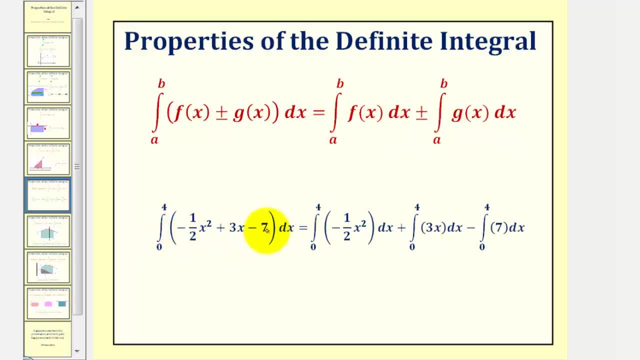 So, as an example, if we're integrating this quadratic function from zero to four because we have a sum or difference of three terms, we can write this as the sum or difference of three separate integrals, as we see here. Next we have the integral of f of x. 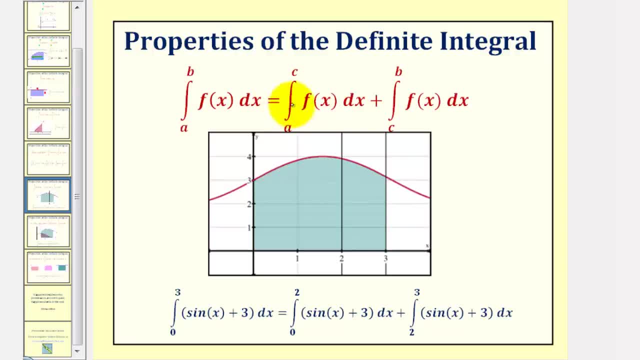 from a to b equals the integral of f of x from a to c, plus the integral of f of x from c to b. To help visualize this, if we integrate sine x plus three from zero to three, again the function is non-negative over this closed interval. 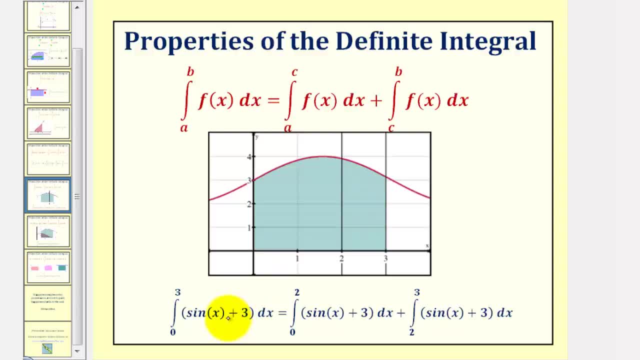 and therefore the shaded region would be the value of the def integral. And we can write this as two separate integrals if we select, let's say, two, If we integrate from zero to two, which would be this integral here, and then we add this integral. 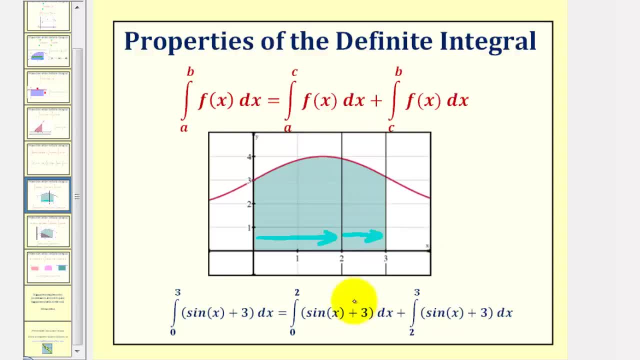 where we integrate from two to three, from here to here, the result would be the same as integrating from zero to three. Notice: in this case, two is the value of c given in this property. In this case, two is in the closed interval from zero to three. 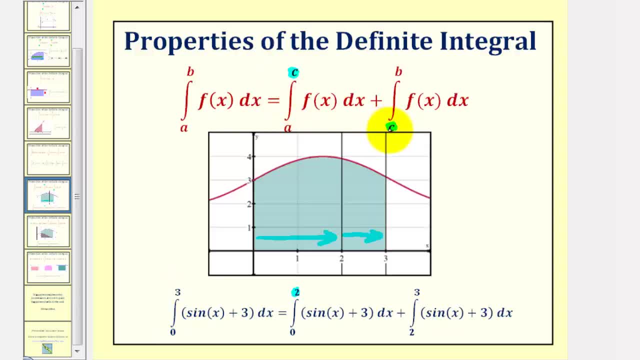 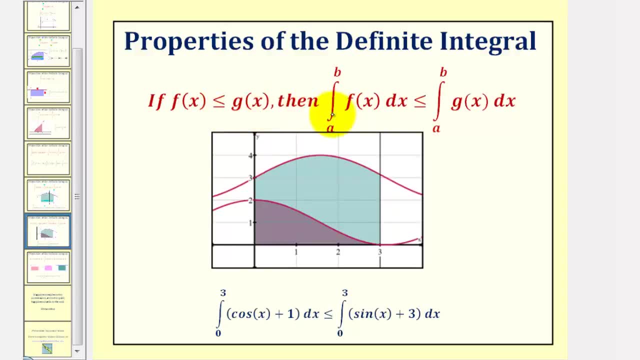 but this property is still true even if c is not in the closed interval from a to b. Next, if f of x is less than or equal to g of x, then the integral of f of x from a to b will be less than or equal to. 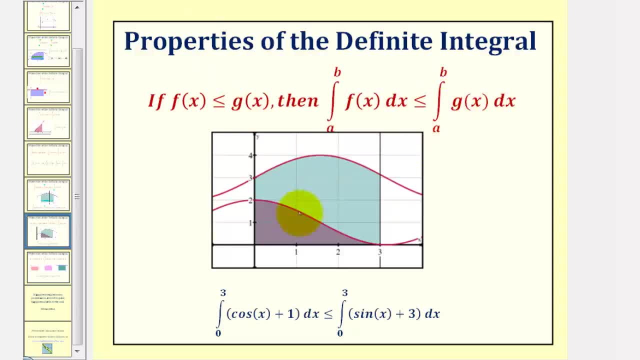 the integral of g of x from a to b. As an example, this function here is: f of x equals cosine x plus one, and this function is g of x equals sine x plus three. And since f of x is less than or equal to g of x, 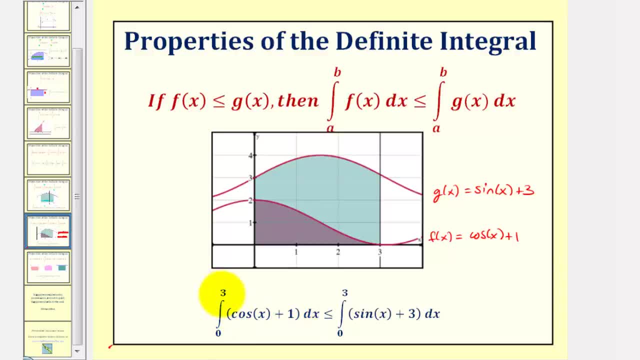 the integral of cosine x plus one from zero to three is less than or equal to the integral of sine x plus three from zero to three, Where, because both functions are non-negative, this integral is equal to the area of this darker shaded region here. 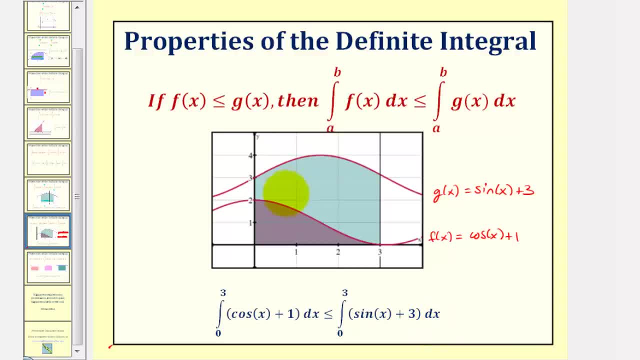 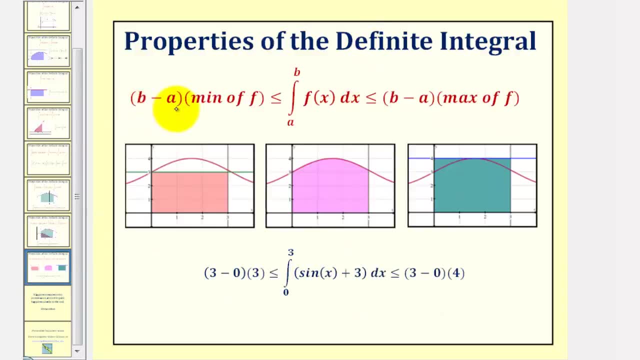 and this integral here would be equal to the area of the combined shaded regions we see here. Let's take a look at one more property. Here we're given the quantity b minus a times the minimum of function f on the closed interval from a to b. 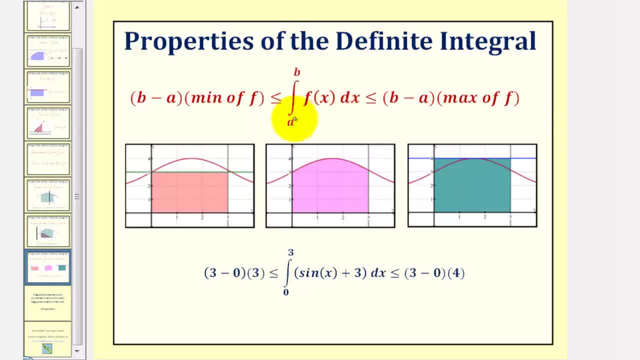 is less than or equal to the integral of f of x from a to b, which is less than or equal to the quantity b minus a times the maximum of function f on the closed interval from a to b. Let's begin by looking at this middle graph here. 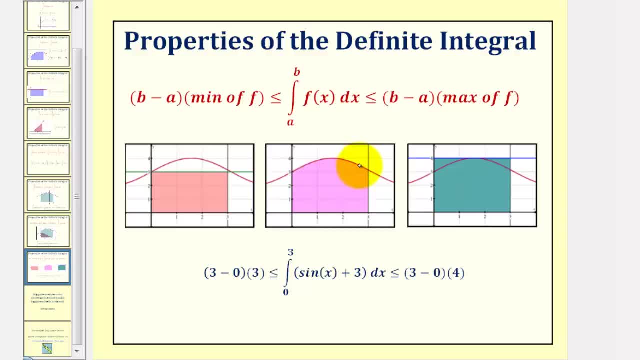 where the function graphed is f of x equals sine x plus three. So because the function is non-negative on this closed interval, this area is equal to the integral of sine x plus three, from zero to three. And now, if we select the minimum function value, 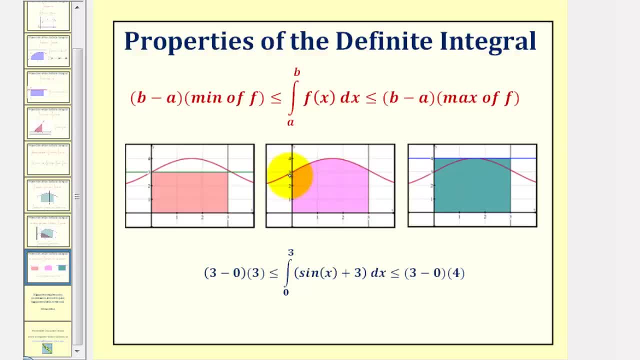 over this closed interval, it would be positive three. So in green we have the graph of: y equals three and the area below this function on the closed interval from zero to three would be the quantity b minus a times this minimum function value, which in this case would be three times three or nine. 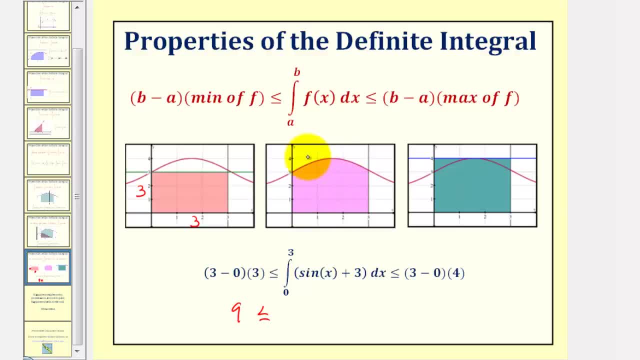 And now the maximum function value of our function f of x is four. So if we graphed y equals four, which we see here in blue, and found the area under this function bounded by the x-axis, because it's a rectangle, we know it's going to be.